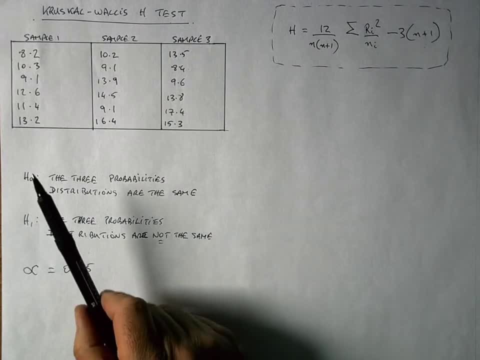 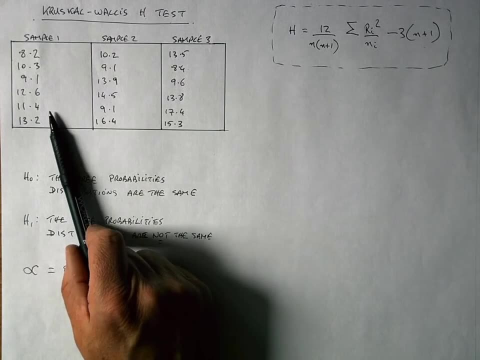 as usual, let's take a look at our data. And Kruskal-Wallis test is a non-parametric version of an ANOVA test and in this case here I'm looking to see if there's a difference between three samples. So I've got sample one data here, sample two data in the centre and sample three. 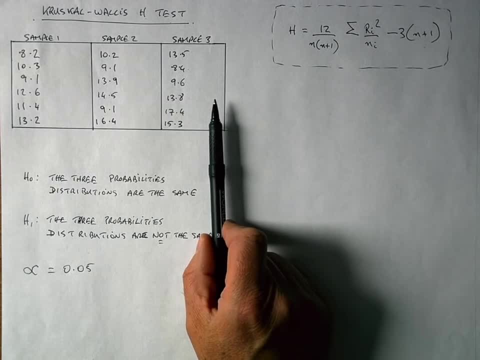 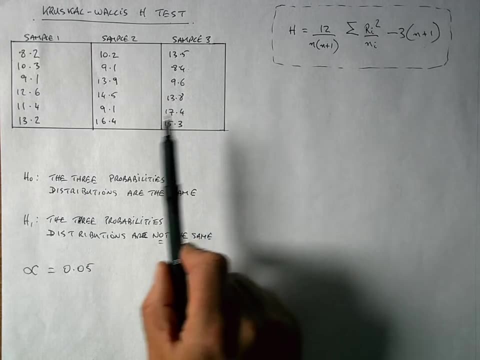 data here. I can use this test for four or more samples, should I choose to do so. Very often with a Kruskal-Wallis test, we're dealing with ordinal data such as ratings and so on, or, as is the case here, we could be dealing with data that are not normally distributed. If they were, we would use. 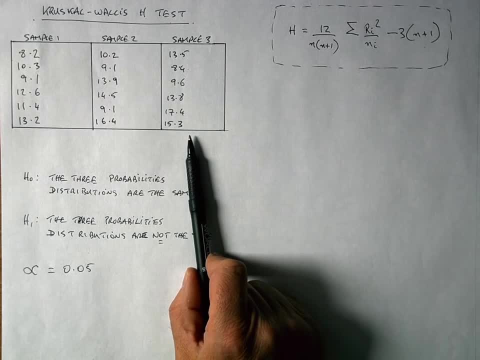 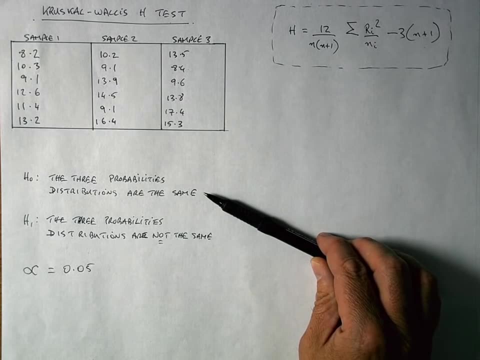 an ANOVA test. so if they're not normally distributed, we'll use the Kruskal-Wallis H test And as it's a stats test, we need to, as always, set out our null and alternative hypothesis. our null hypothesis in this case here is that the three probabilities distributions are the same. 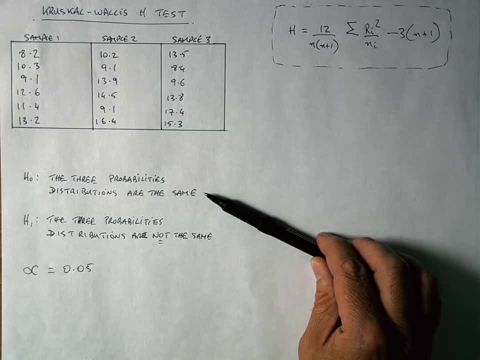 in other words, there's no difference between sample one, sample two and sample three, And our alternative research hypothesis is that the three probability distributions are not the same. in other words, at least two of them differ, And in this experiment here. 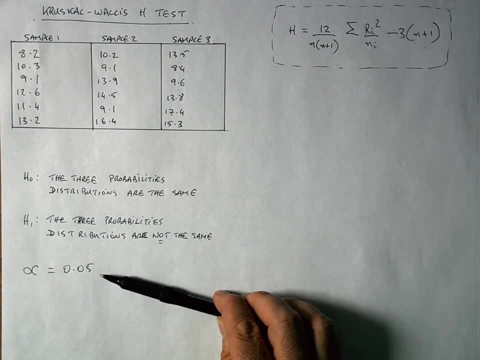 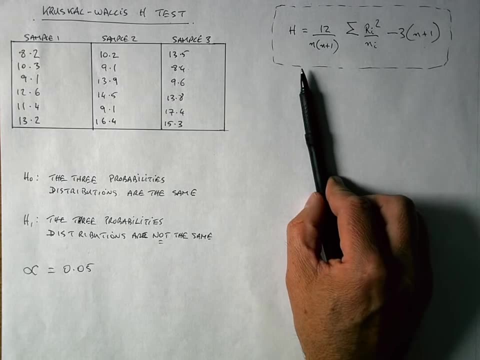 our calculations we're going to use a significance level at an alpha value of 0.05.. Now a formula for calculating the H test or the H statistics looks a little bit awkward at first, but when you read through it it's relatively straightforward. 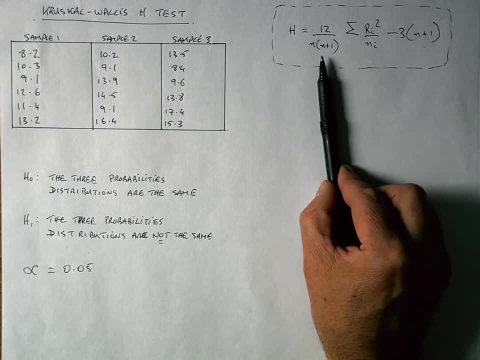 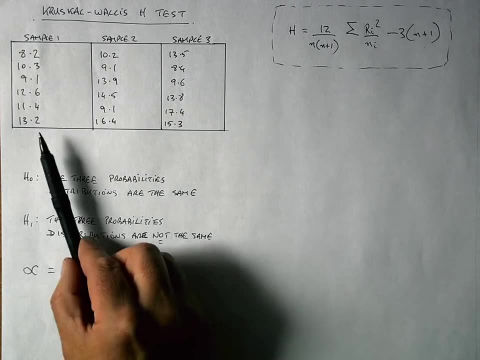 to work through. So our H statistic is equal to it's in three parts. So this first part here is 12 divided by n times n plus 1.. Now n is the total number of values. So in my case here I've got 6. 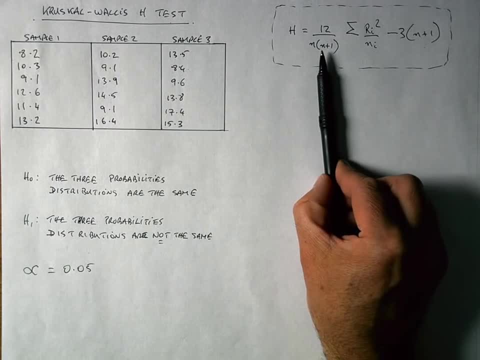 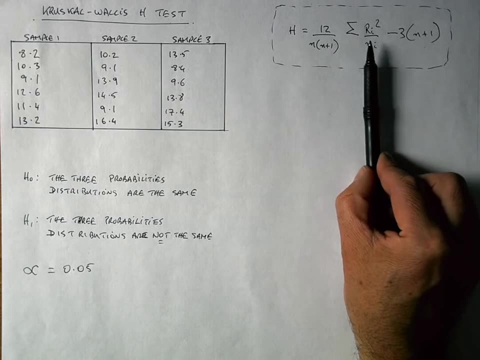 plus 6 plus 6 values, which is 18.. So n is going to be 18 in this version of the formula. The business bit of this formula is the bit in the center. here We need to sum up r, which is all the ranks, i for each numbers of groups. So I've got. 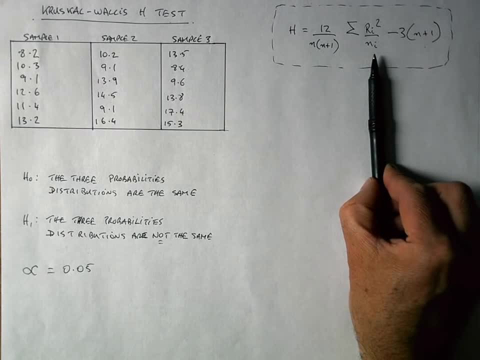 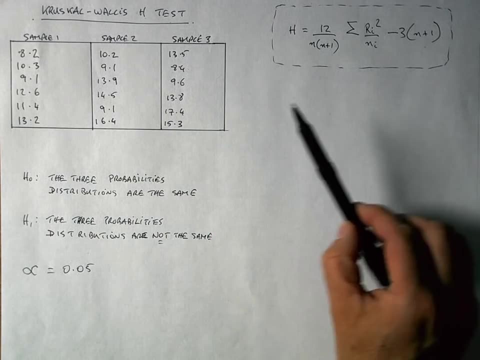 groups. so we're going to do this three times and we're going to divide that by the number in each group, and it happens to be six in all cases here. so i've got six in sample one, six in sample two and six in sample three. so i'm going to be doing this three times and then adding up the three. 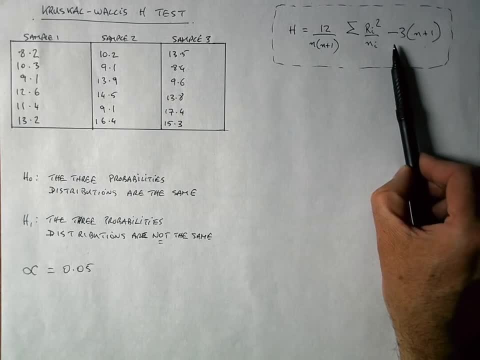 values for this bit in the middle. and then the final part here is: we're going to subtract three times n, which again is 18 plus one. so be just be careful here when you're doing this, to distinguish n, which is here, here and here this is going to be 18 in my example, to distinguish that from ni. 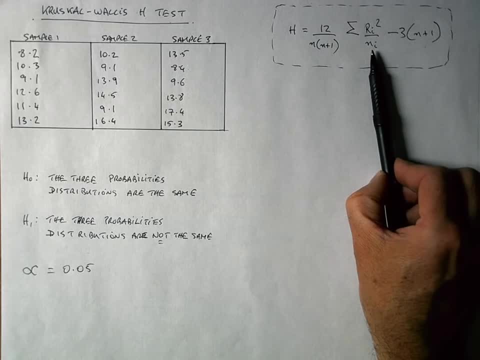 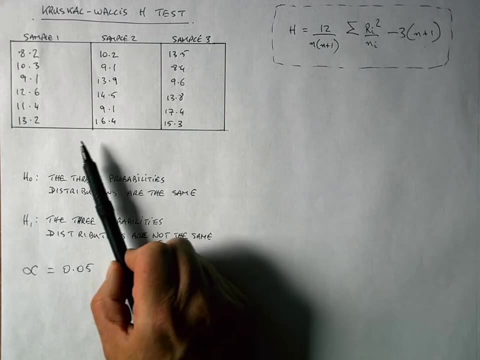 which is the number of values in each group or each sample. now, the good news about a Kruskal-Wallis test is, if the data that are here, you don't actually do anything with it at all. you're not going to calculate the mean or standard deviation or variance or range or anything like that. 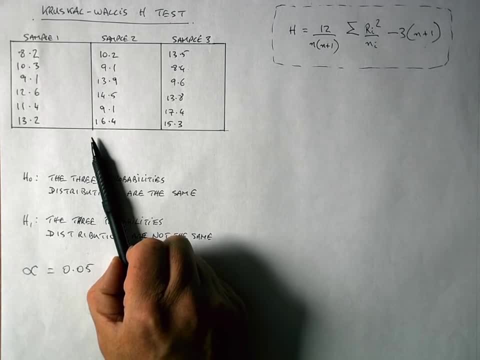 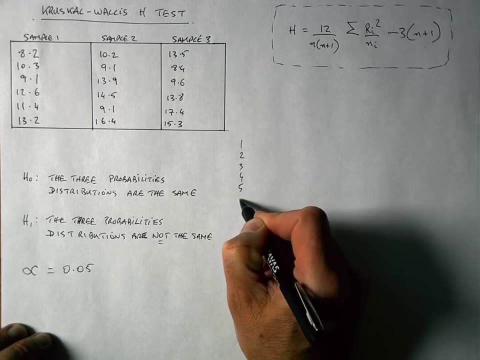 but we do need to rank these data from the smallest to the largest. so my first job here- is i'm going to do this here- is to write out, from 1 to 18, the numbers to represent the ranks of each of my data here. so you 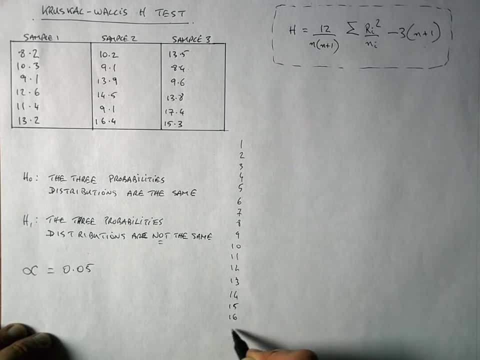 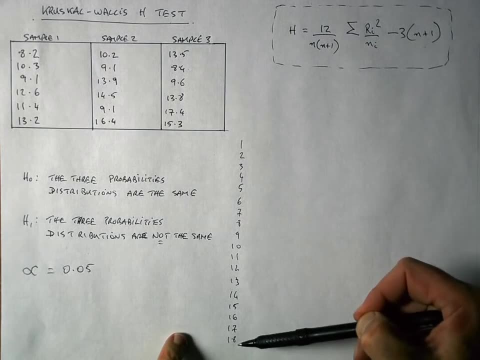 could do this in excel or on paper, like i'm doing it here. so i've got 18 values here and i'm going to rank each of these numbers here so that they match up with with a rank from the smallest to the largest. so i'm going to work through my data and see which value is the smallest, and as it. 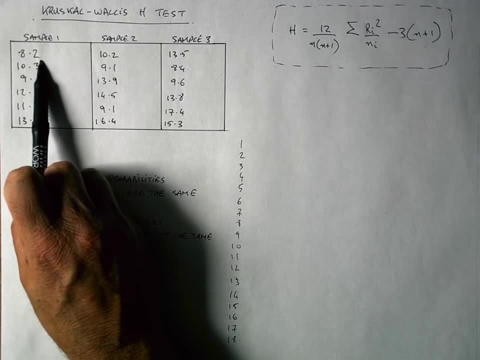 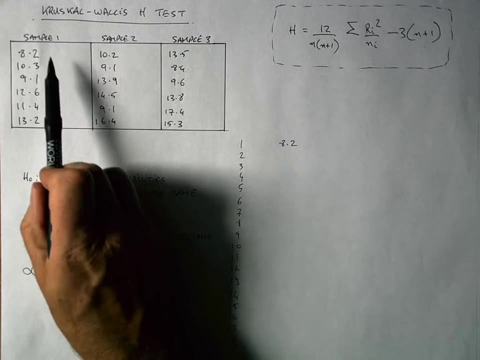 happens. the first value is the first value in sample one. so the first and lowest value for ranking number one is 8.2. so i'm going to write that here, beside number one, my next lowest value. as i go through them all, i can see that it is. 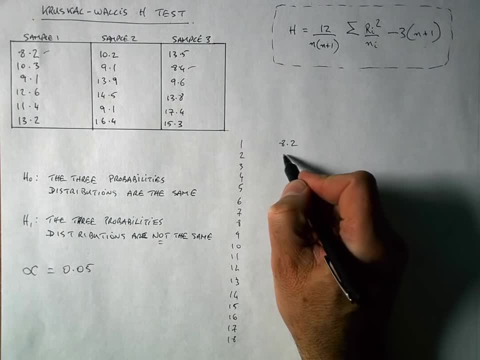 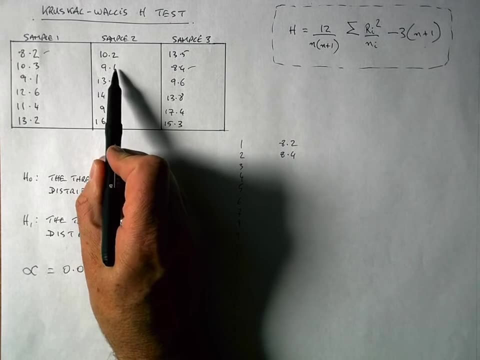 8.4. so i'm going to tick these off as i'm going along. 8.4 and then my next lowest value: as you can see, i have a 9.1, but i also have another 9.1 and a third 9.1. so tick those off. so i'm going to have. 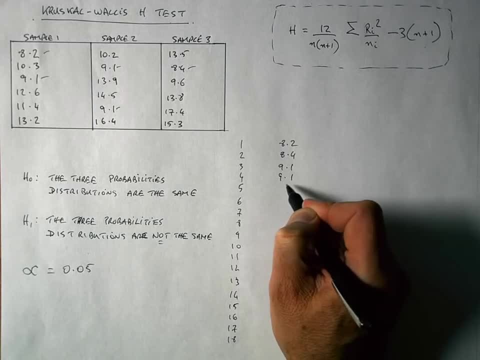 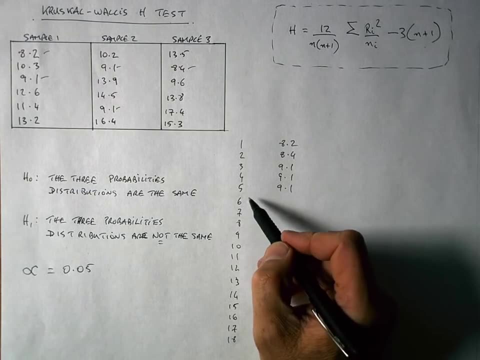 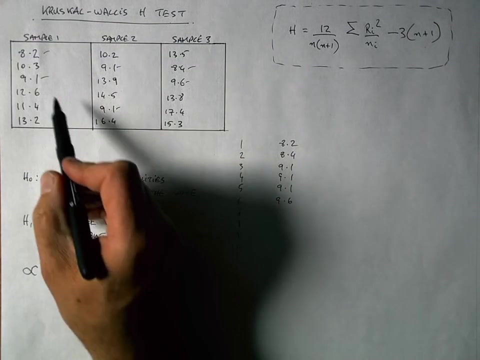 rank number three, 9.1, rank number four, 9.1 and rank number five, 9.1. that represents a tie which we will come back to in a few moments. my sixth lowest mark is a value of 9.6. next one then goes on to 10.2, which is up here. i'm just going to quickly fill on in all of these. 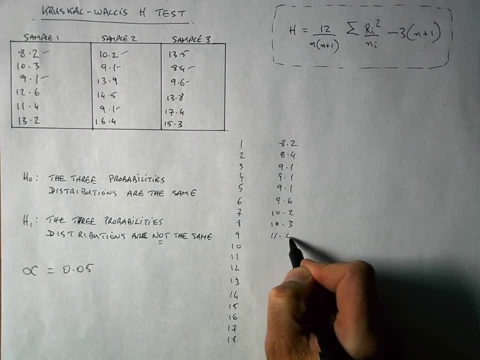 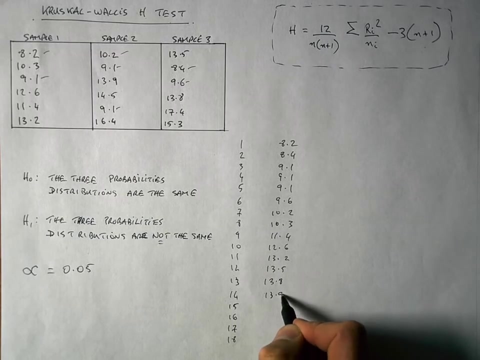 you can work these out yourself for any sample data that you are doing, just making sure at all stages that you don't skip any values and watch out for times. in my example here i do not have any more times and 13.8, 13.9, and you know, tick these values off as you're going along. i'm just 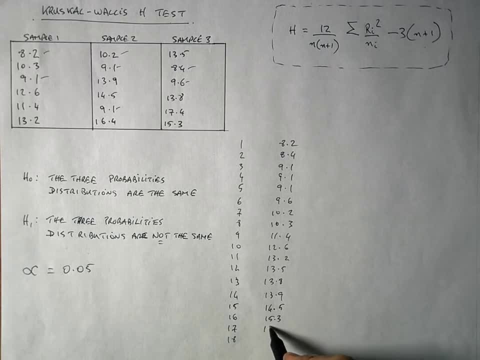 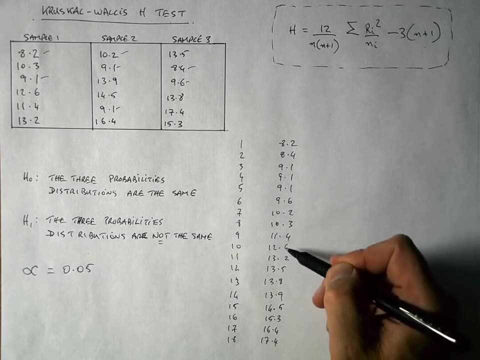 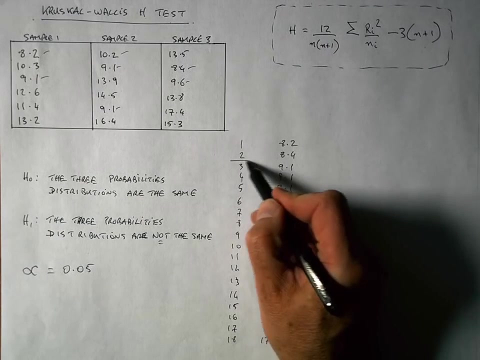 trying to keep that times sticker tight. so that's all that it is. and then my second highest value is 11.2. so this is going to be the highest value of the other three values i'm going to use for illustration purposes. and the final and highest value of all is 17.4. so when you've done this, 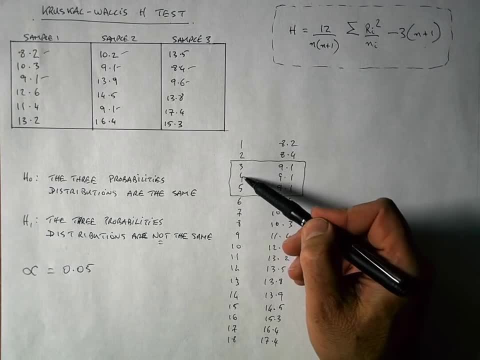 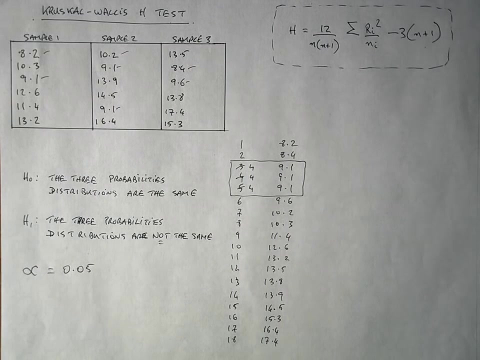 please make sure- and recheck all the values- that you've got the rankings correctly, because it's the rankings that you were going to use. now, as i mentioned, we've got a ties here in this section. 5 is 12, so dividing those up by 3, I will get rankings of 4, 4 and 4 here. so I'm 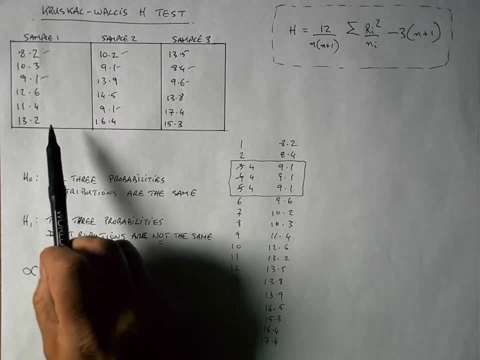 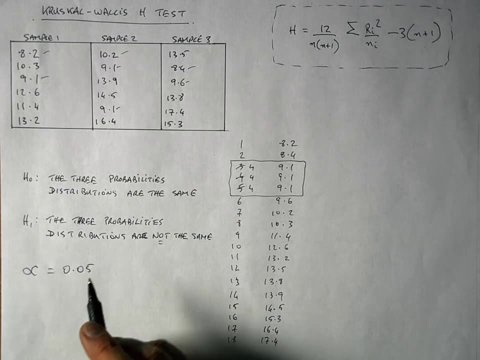 now ready to add these rankings to my table over here, and you notice that I've left some space at either side of my columns of data here so that I can write in the ranking for each one. so now I want to put the rank here. rank and rank. so 8.2. go down to my list here, see where's 8.2, and I can see that that ranks as number one at 10.3. I'll have to look down to this and see where 10.3 is that ranks as as number eight. so take that one off there: 10.3, that's right. 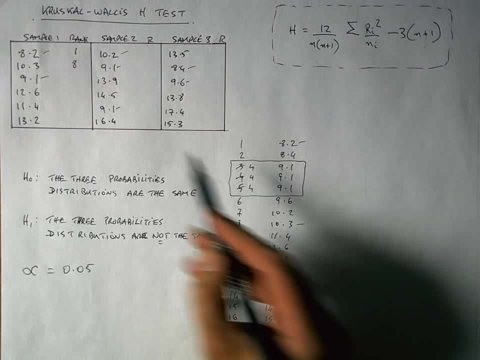 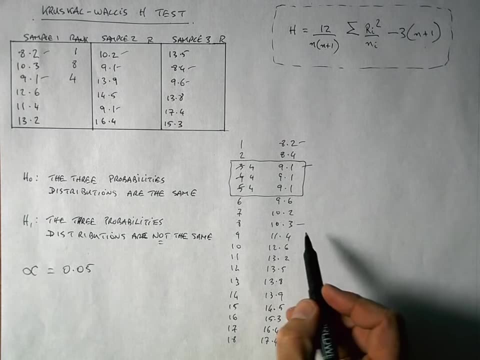 number eight. the next one is one of my ties. nine point four. so I can see they're all ranked as four, so I'm gonna put it. use one of the fours there. twelve point six: if I go down to here, I can see that that's ranked at number ten, so right. 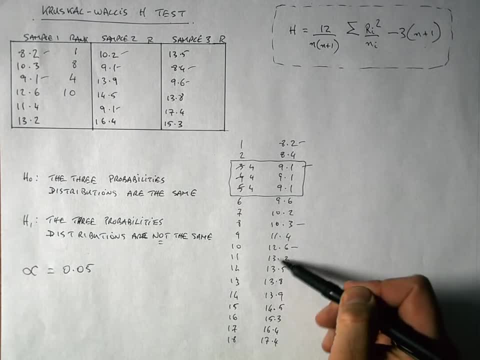 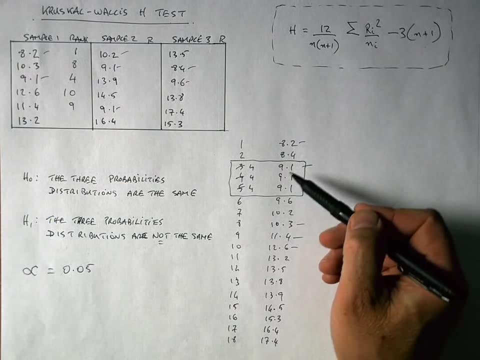 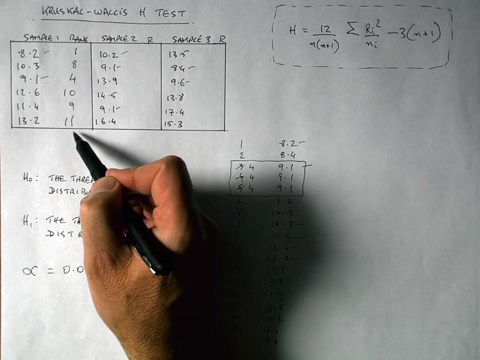 in ten here. eleven point four go down to my list. there's eleven point four. it's ranked as number nine and finally, for the sample number one, the thirteen point two. if I go down to here I can see thirteen point two is ranked as number eleven. so I've got all the ranks for sample one and then I go in and I do. 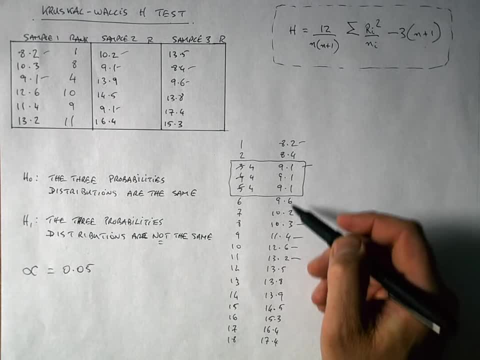 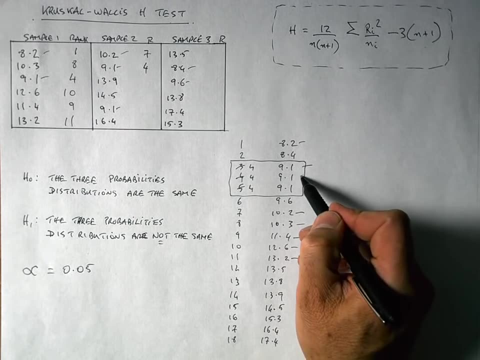 this for sample two. so sample two. very quickly. ten point two go down to my list. I can see that that ranks as number seven and nine. point one is another one of my ties and again I put in number four in here, crossing off one of the nines, and I'm just going to quickly work down through. 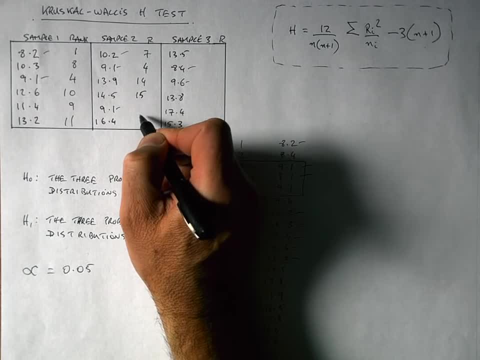 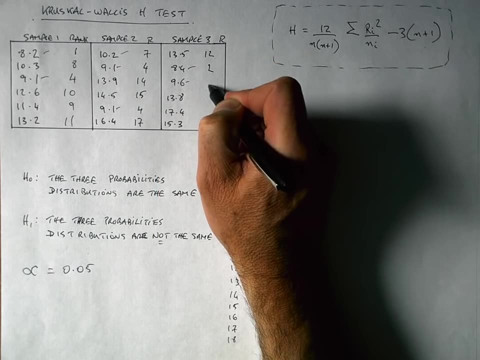 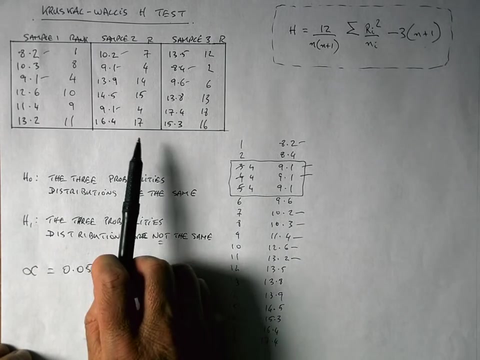 all the rest, as I've got them all prepared here: fifteen, four and seventeen, and then go along. do the third sample, which was the ranking of twelve and two, six, thirteen, eighteen and sixteen. again that always recheck all your data to make sure that you have made the right rankings beside the right values. now 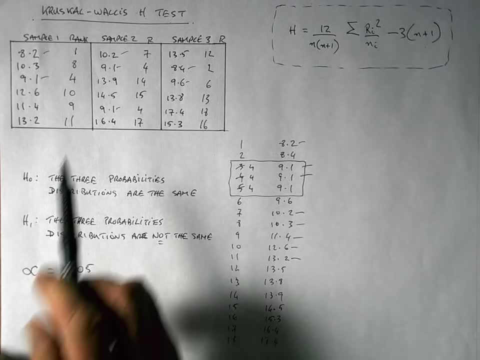 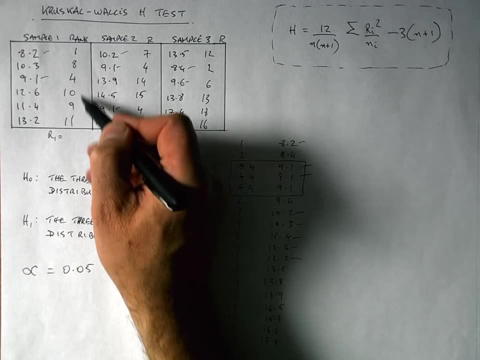 it's time to do some calculations. we need to sum up each of the rankings for each of the three samples. okay, so I'm going to call the sum. here are one for the sum of the ranks for number one. when I add up these six values here, I get a value of 43. I got to. 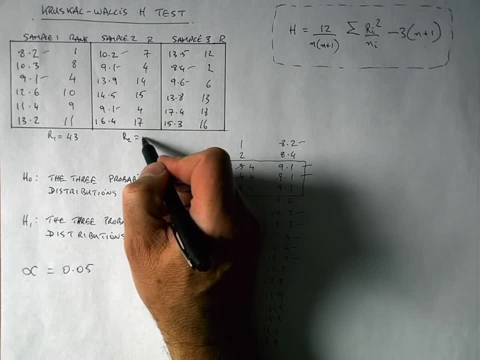 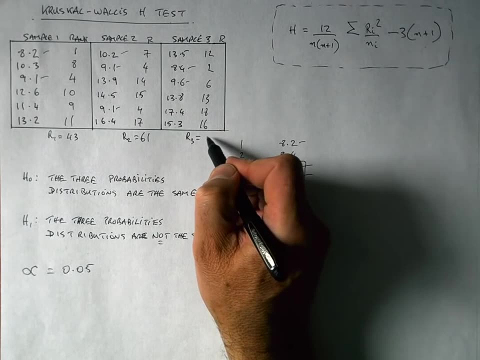 sum up the values here for R2, and that's when I add all those up, I get a value of 61. and finally, when I sum up the ranks for a sample three called R3 that's, I get a value of 67. so that's the first bit of the. 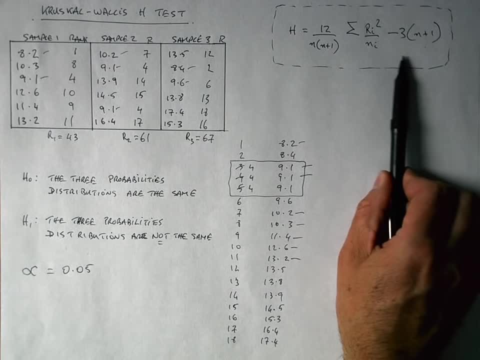 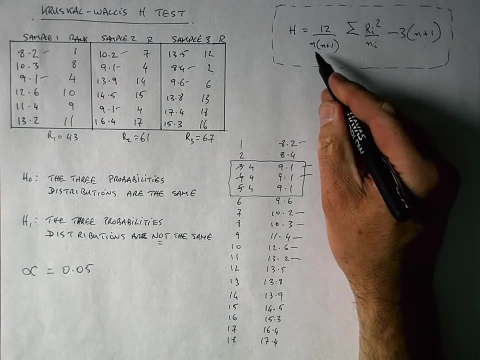 computing done. the next bit, then, is to put my values into my formula over here. so let's rewrite my formula out here. so the H statistic is equal to 12 divided by n, which I've already determined is 18, the number of values multiplied by 18. 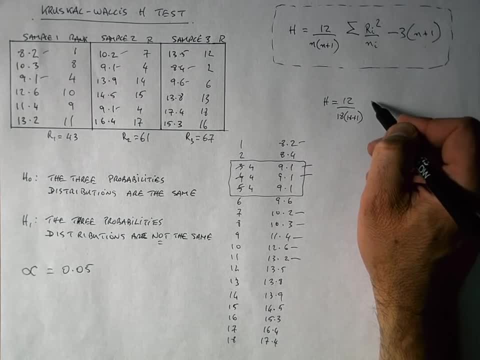 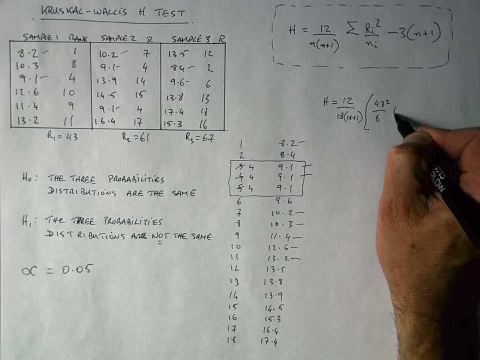 plus 1, and then I'm going to add to that. multiply that by the sum of each of my three sets here. so R1 squared is going to be 43 squared divided by the number n in sample, the first samples, but that's going to be 6, and then I'm going to add: 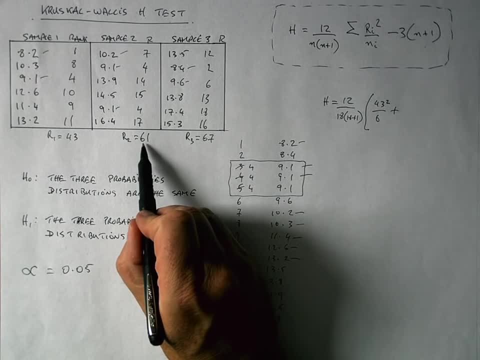 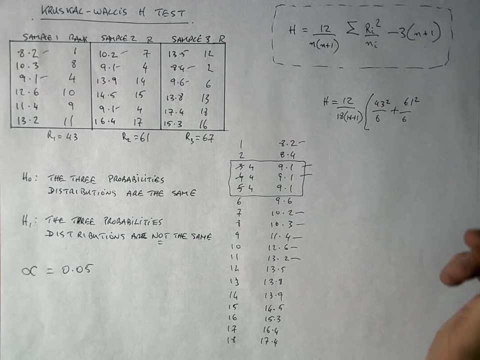 that, because I'm summing here, don't forget- to R2, which is 61 squared. divide that by 6 again, because I've got six values in sample 2, and finally add that then to the sum for rank 3, which is 67 squared divided by 6, and we multiply. 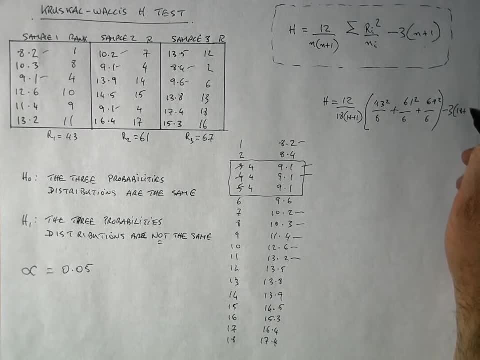 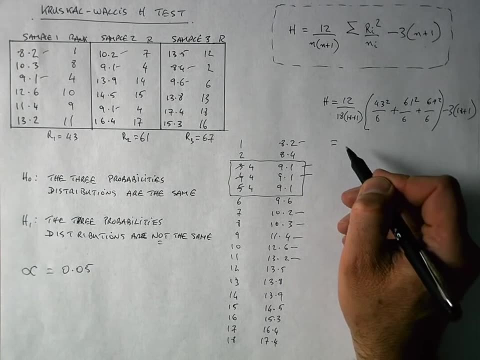 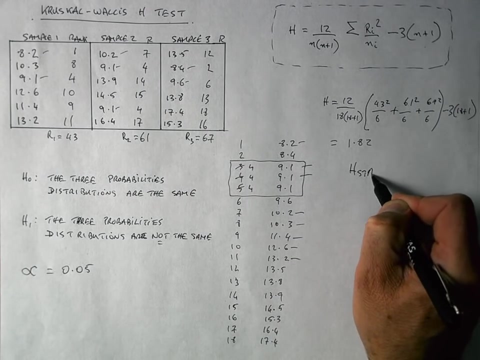 that by minus 3 times 18 plus 1. okay, so follow back through there if you're not sure where each of these values came from. and when I work all of that out, I get a result of 1.82, so my H stat is equal to 1.82. before I can determine. 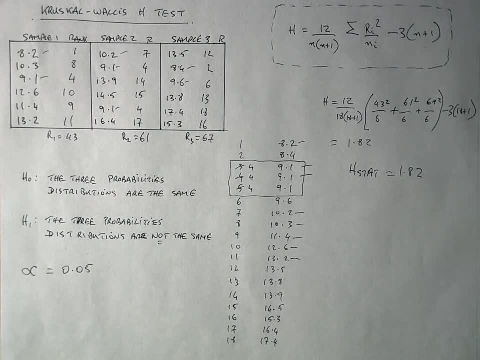 whether this is a significant value or not. I need to determine the degrees of freedom, so I'm going to abbreviate that as degrees of freedom at DF, and it's very simple calculation. for a Kruskal-Wallis test, as in a one-way ANOVA, it is the